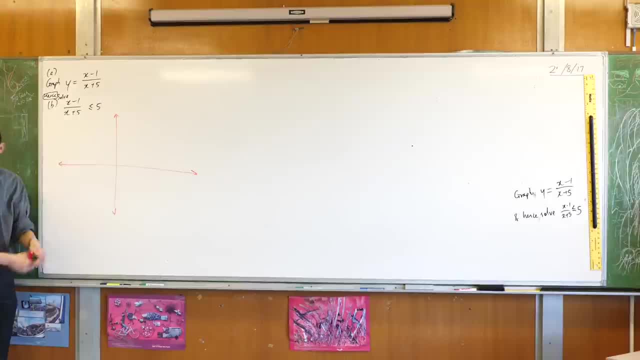 graph that can possibly fit all of the features that you've got. okay, The guide that I've given you before still applies for something like this, but it's quite simple, So, in fact, you'll find we don't even need to go through all of. 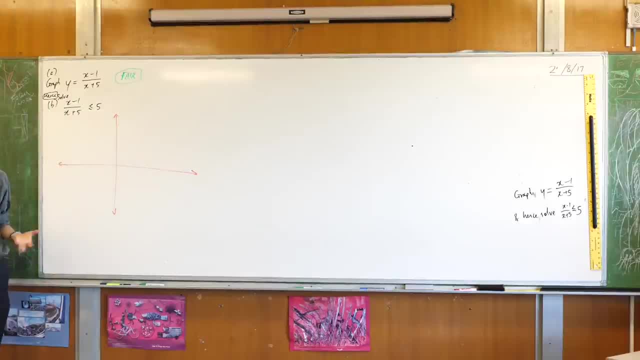 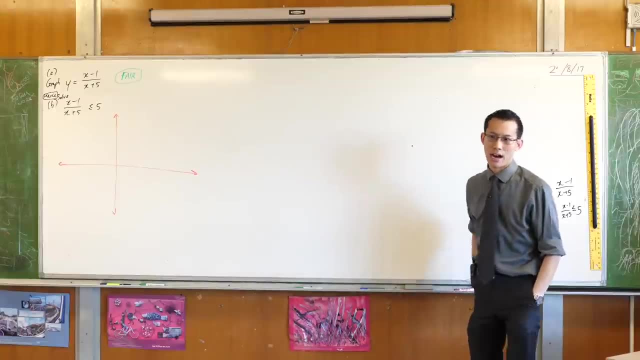 these steps before we've got enough of a picture to know what the graph looks like. So what does F stand for? F stands for factorized. In this case there's not much to do, And in two unit you will frequently get graphs that are so simple. 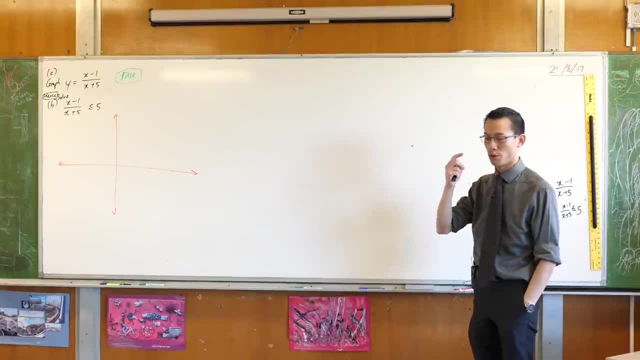 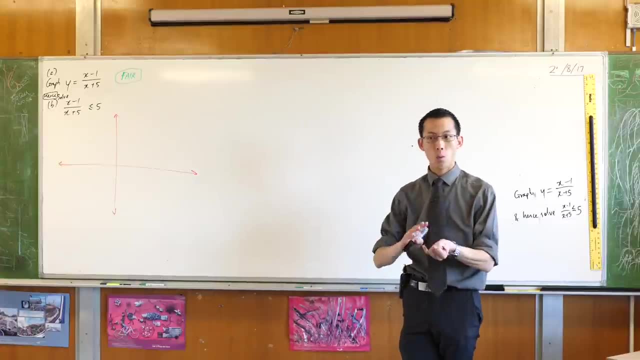 there's not really any factorizing required, but the principle helps you with tougher questions. The next question is asymptotes. Now you guys know there are two categories of asymptotes. One comes from the denominator. What kind of asymptote do we get from the denominator? 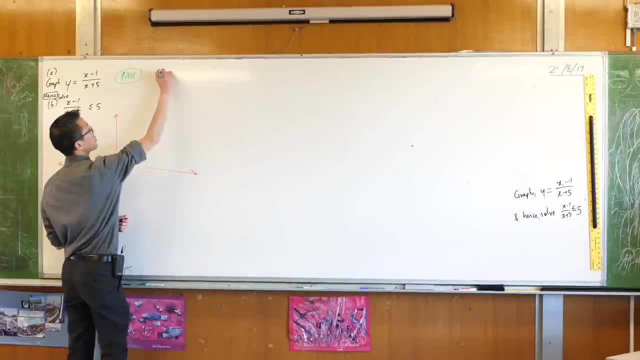 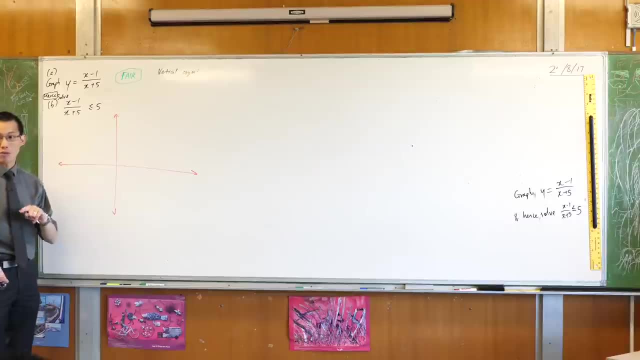 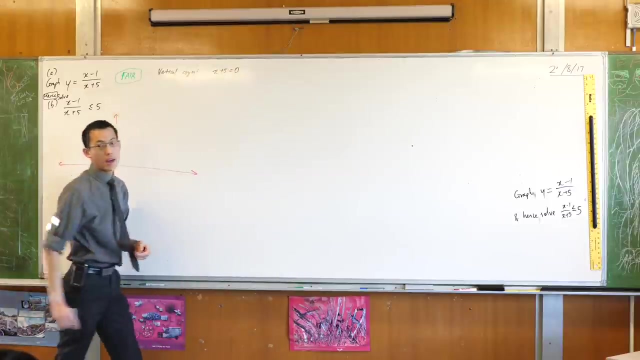 Yeah, vertical ones, right. So what we want? Vertical asymptotes. Vertical asymptotes occur when the denominator is zero, because that blows up the equation, right? So if I say x plus 5 equals 0, right, you get a vertical asymptote, because it's outside the domain. I just rearrange, I change and make x the subject. 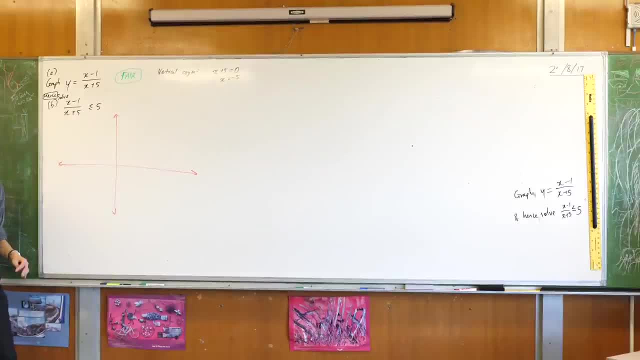 So x equals negative 5 is where I'm going to find my vertical asymptote, So I'm going to draw that in over here on the left-hand side, x equals negative 5.. Cool, That's not the only kind of asymptote. There's not just vertical ones. 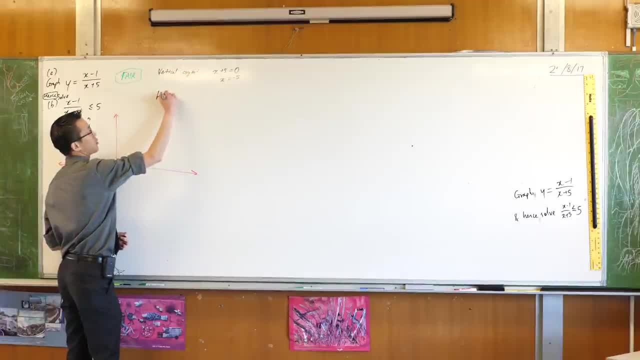 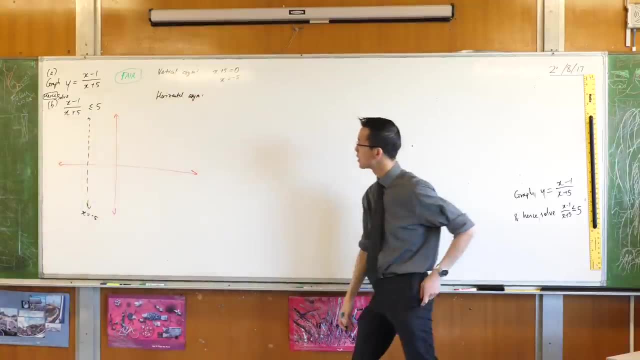 There's horizontal ones as well. right And later on in the course you'll encounter horizontal asymptotes that are off at an angle. We call them oblique ones. We'll come to them a bit later, In two unit. you'll get these, though. A horizontal asymptote is not about the denominator on its own. 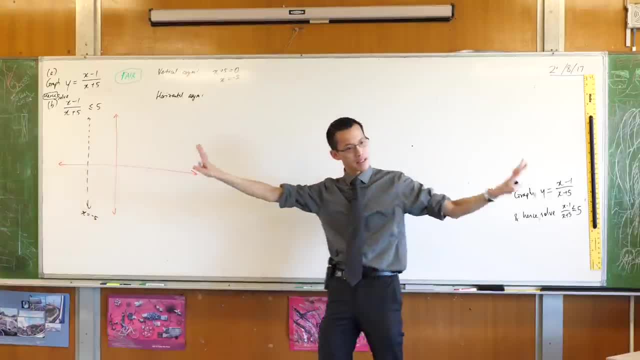 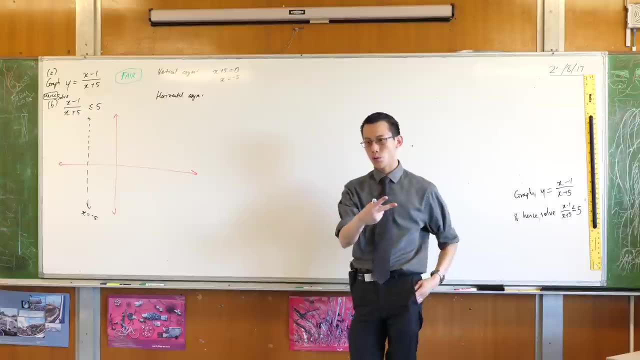 It's about the whole function and what it does at the opposite ends of the graph, Like at negative infinity and at positive infinity. okay, So I'm not sure if you remember this, but it's worth revising. There are two easy ways. actually, there's more than two. 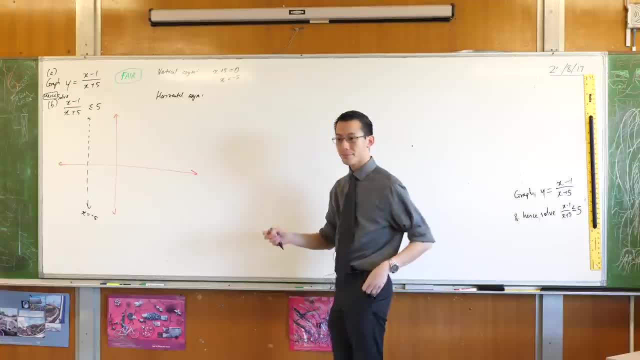 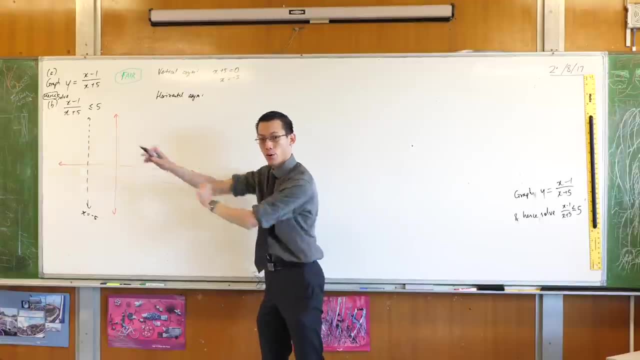 but there are two pretty straightforward ways to find this okay. The first is get your calculator out, grab your calculator and then just test out really big negative values or really big positive values of x. So, for example, you could test: x equals a thousand. 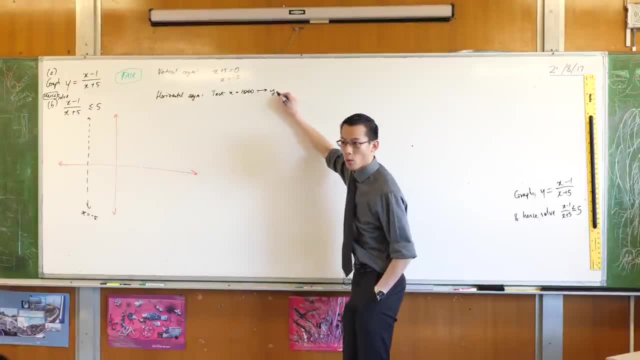 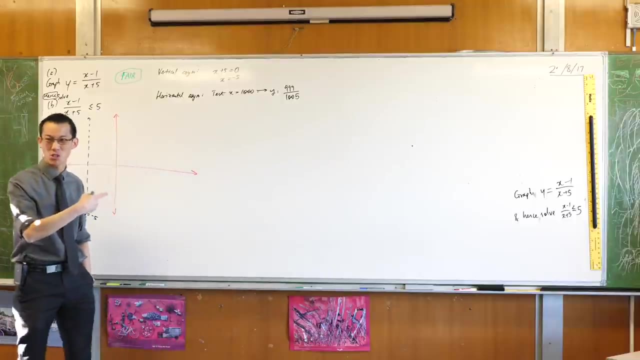 right. If x equals a thousand, then y will equal. what's on the numerator- wait, numerator 999, and your denominator will be 1005.. Now you can get your calculator to turn that into a decimal if you like, but clearly that's close to one right. You also want to. 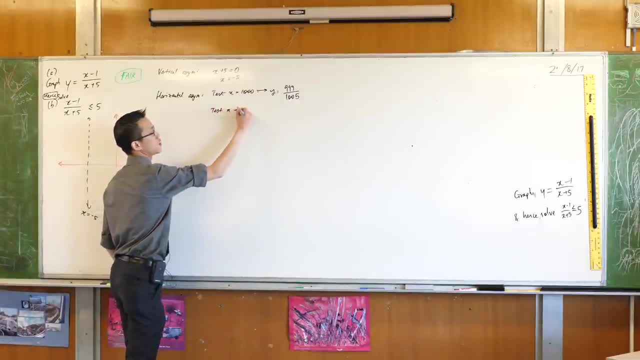 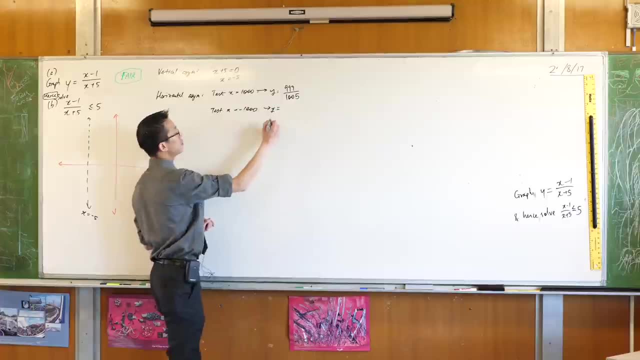 test the other side, just so you make sure you know what's going on. If you test, x equals negative a thousand, so I've gone to this end right. negative. then y is going to be equal to. let's have a look. 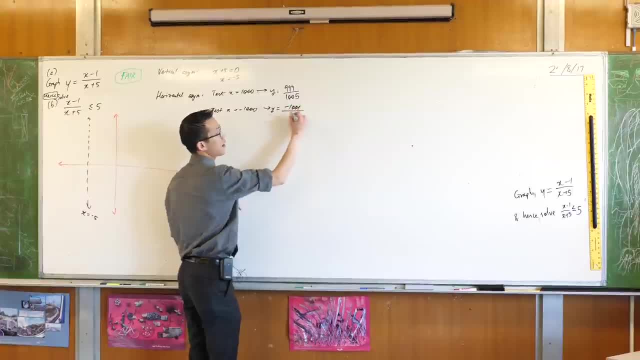 negative, a thousand one divided by which, if you notice there's two, there's a double negative. so that's just this. Your calculator will also help you see. in fact, I'm going to ask you guys to help me here. 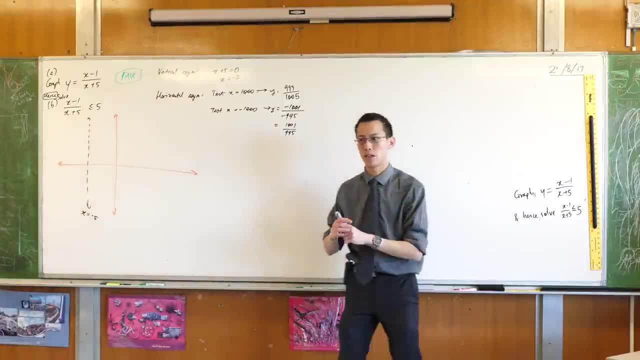 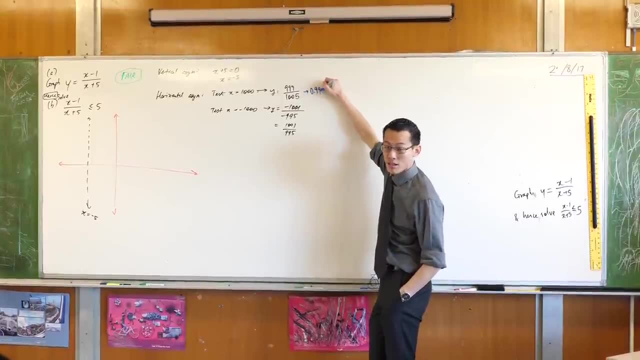 can you give me the decimal values for these guys? Just give me a couple of decimal places. What's this Zero point 993, yeah, that'll do dot, dot, dot. and what about this one? What's this decimal? 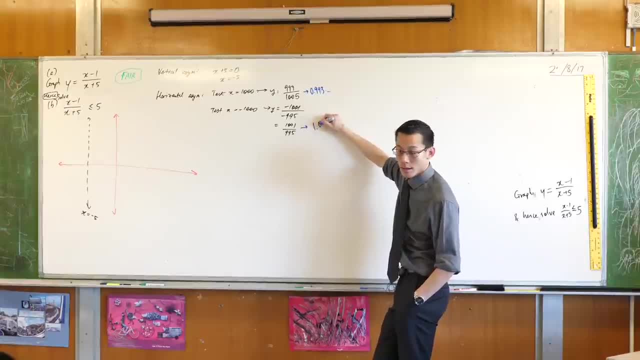 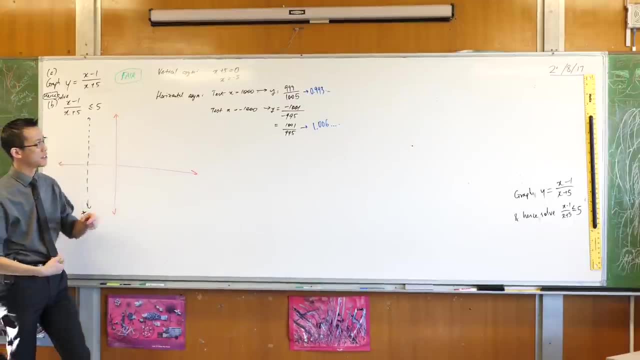 Zero, point 993,. yeah, that'll do dot dot dot. and what about this one? That's one, that's one, zero, zero, zero one. Cool dot dot dot. okay, Now, the only reason why I point this out is because you can work this out without the calculator. but do you see? this is just below one and this is just above. so that's going to be helpful when I draw this thing, okay. 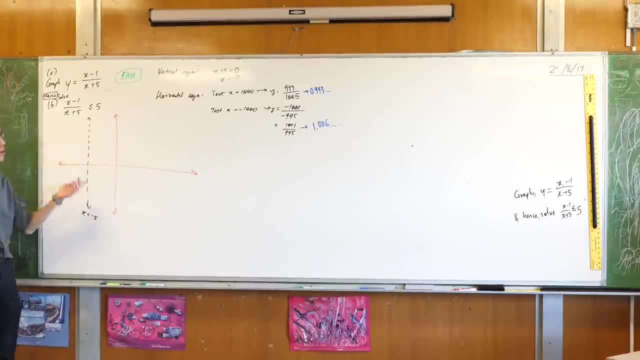 So I've already decided that I've got a vertical asymptote. now I know there's also a horizontal asymptote. it's going to be x equals one, so I'm just going to draw that in. I did say, though, that there's two pretty straightforward. 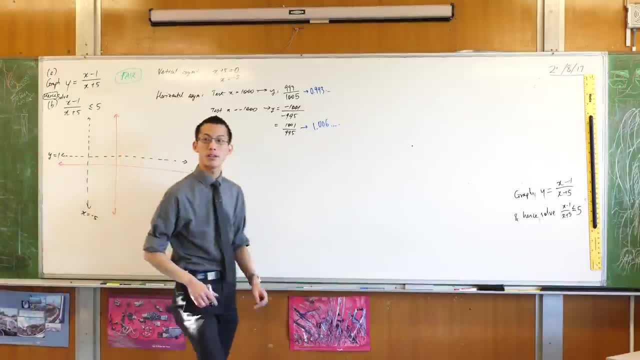 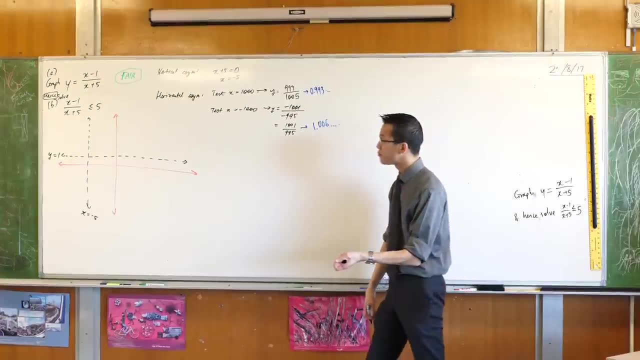 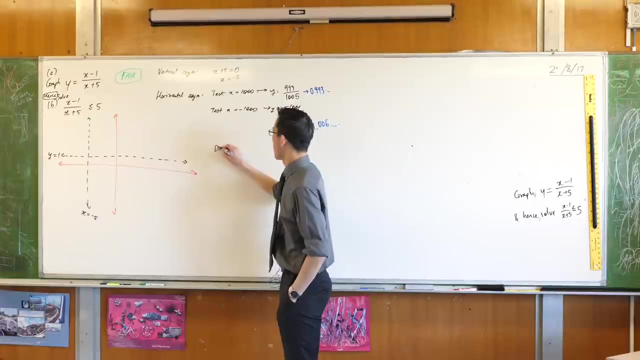 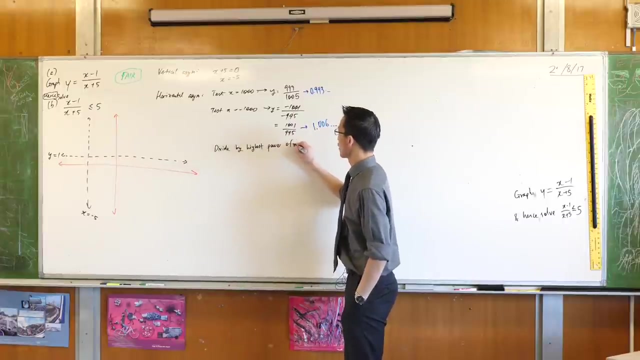 y equals one. sorry. two pretty straightforward ways to work this out. if you don't want to, if this looks a bit inelegant and blunt instrument to you, like I'm just testing values, another thing you can do is take your function and divide the top and the bottom by the highest power of x. let me say that again: divide by highest power of x. so if, for instance, you had x squareds on the top and the bottom, you divide by x squared, in this case, the highest power of x. 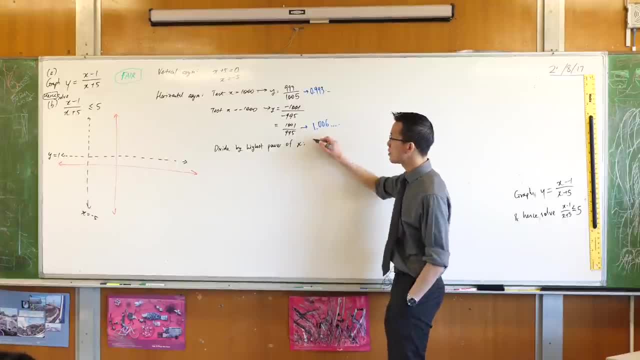 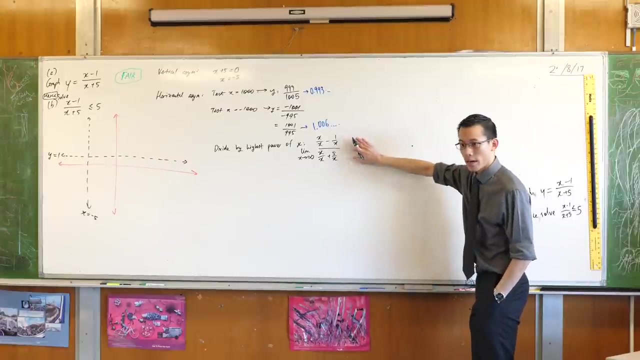 is just, it's just x. so when I do that, I'm going to get x over x minus one over x, divided by x over x plus five over x. see, that, does that make sense? Now, remember, I said: oh, I'm interested in the extremities, right, the far off spots, so I'm going to use my limit notation to indicate that, as x approaches infinity, what happens to this thing? 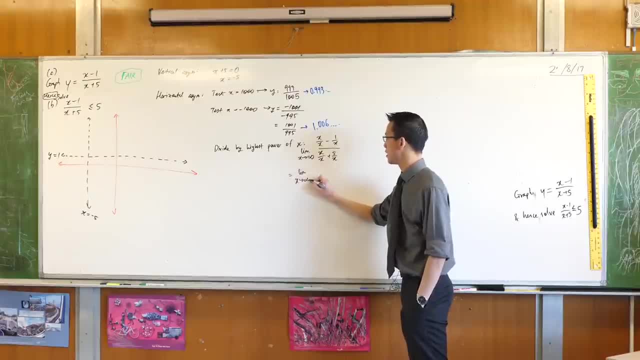 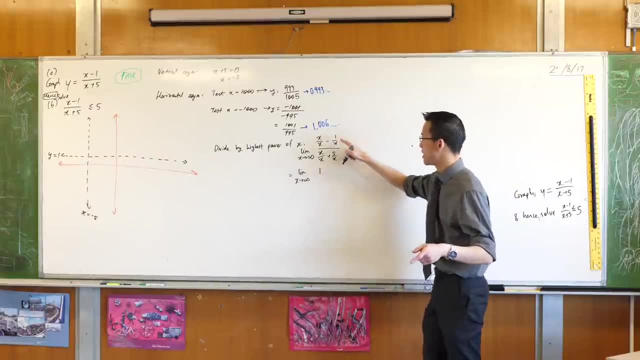 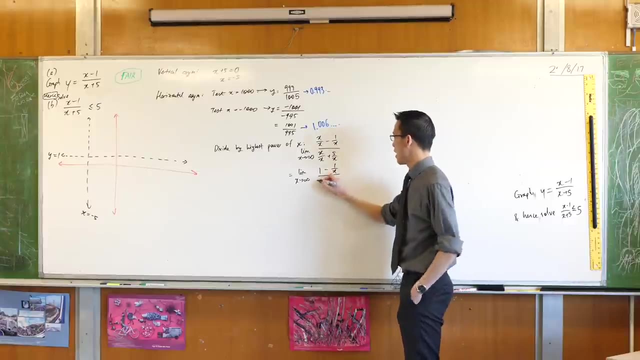 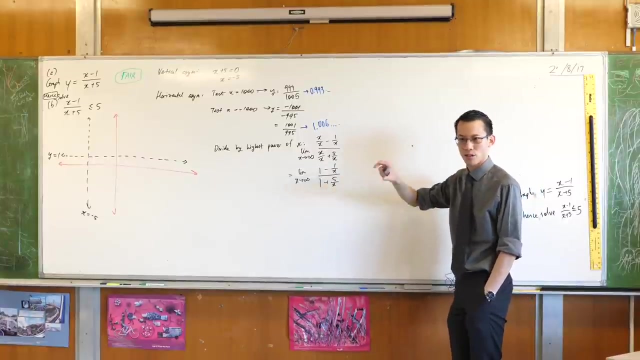 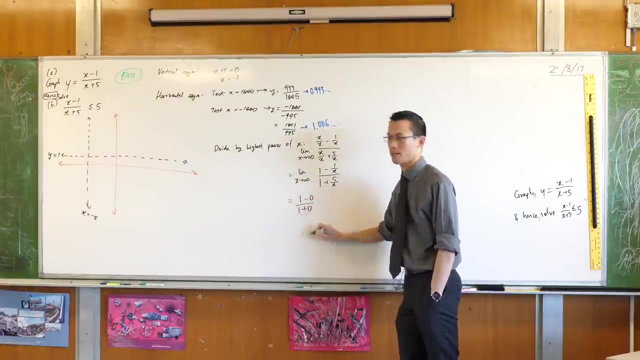 Well, it's going to be. x approaches infinity. These x over x's are just wait hold on. x over x's are just one. but these guys here, yeah, they're going to get tiny because it's one over some ridiculously large number. this guy over here is five over a ridiculously large number, but because it's ridiculously large, he doesn't care. the five just sort of vanishes away. okay, so you can see, here this is going to become one minus zero on one plus zero. 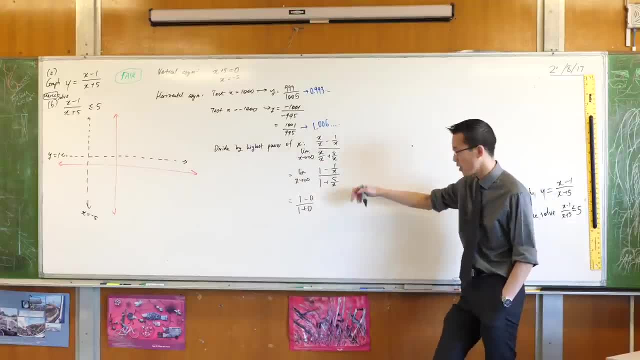 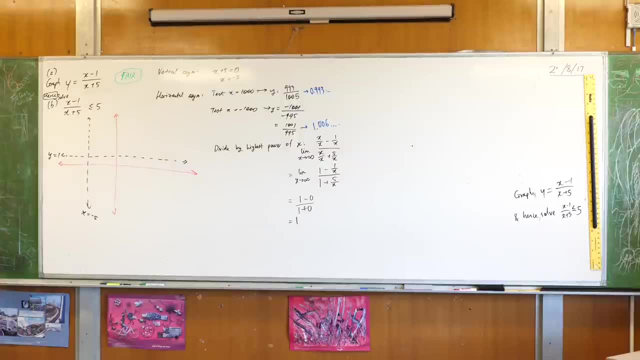 so those, those, those terms there are insignificant and, just like we got before, we're approaching one okay. okay, do you mean like this? the ridiculously large number is anything I like, so I put in a thousand because that's large. you can put in a million or ten million if you want. it just becomes a bit silly and pointless because you're already getting this behaviour very obviously right for this one here. 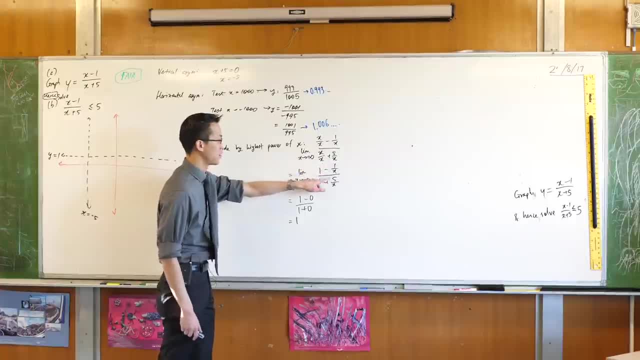 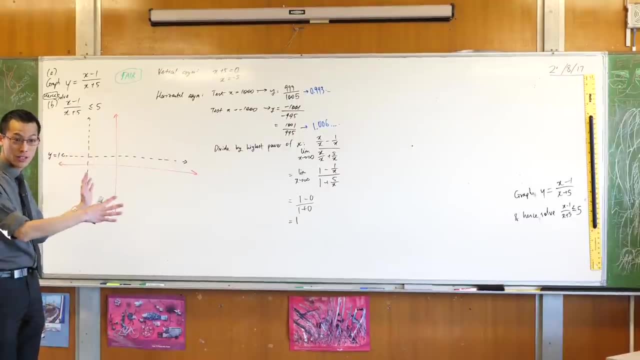 so I've. I've tested out as x approaches infinity, right? so therefore these things are going to clearly vanish. okay now? by the way, I did say I'm with you this whole time. Rokal's going to come in here, so I'll finish this, because I'm almost there, and then we'll let them come in and do their thing and then we'll come back, okay, if you guys want to. 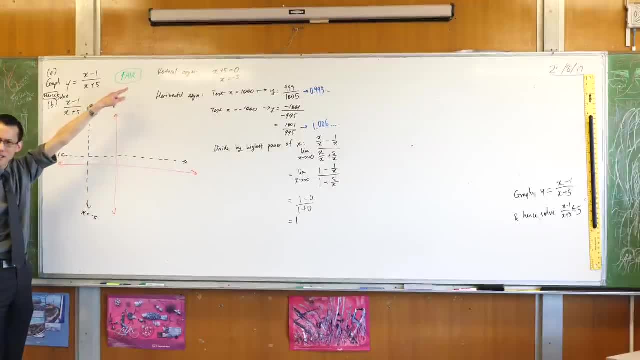 All right, factorised. I've got asymptotes. i stands for Intercepts, very good, so you guys can quickly tell me when x equals zero. when x equals zero, watch what happens. you just get left with Negative one over five. so I'll put that guy there. and when y equals zero, when y equals zero, that just means the numerator has to be zero, right? if the numerator is zero, the whole thing is zero, do you agree? 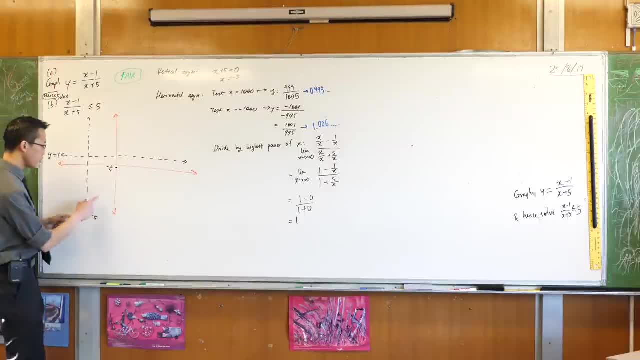 So then the x value that gives you, that is, x equals one. keep in mind this is negative five or a distance of five. so I need to make sure my scale is somewhat consistent. so I'm going to put one about there. I'd say: 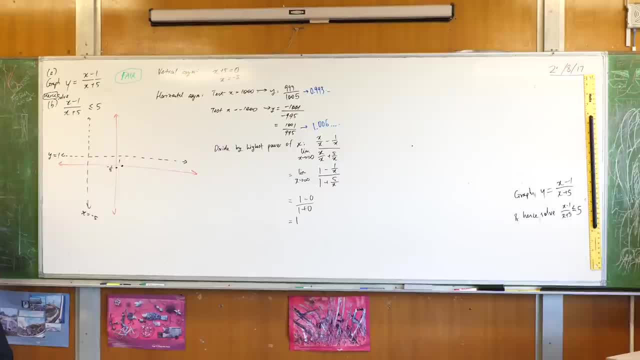 Okay, now, if you wanted to, you could then go and do regions. but it's fairly straightforward when you have a look at this that it's going to go from positive because you've got two negative factors, then down to negative, then to positive. you can draw that in if you like, but this is so simple and you can see, for example, you've got to pass through here, you've got to go toward, but just below this asymptote, so it's going to look like I'm going to have to do this kind of thing. do you see that? so 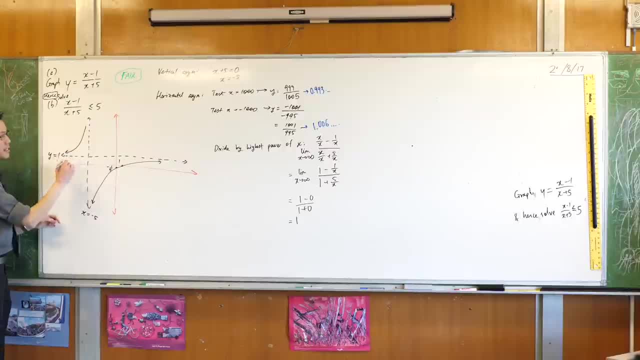 here we go like so and over here, remember, it said: we're going to end up just above that. y equals one line, so that's why it doesn't like: sneak down underneath, and that's it. that is the shape, okay. 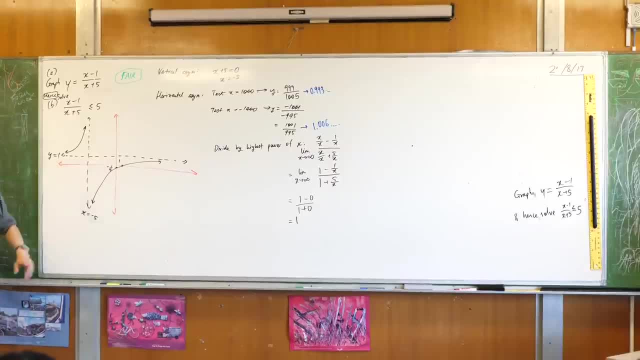 Okay, now lastly, less than or equal to five. okay, what I would do here if it says hence. if it says hence, I'm just going to put in five onto this graph. where would five be? well, there's one, two, three, four, five. sorry, my scale's not great. 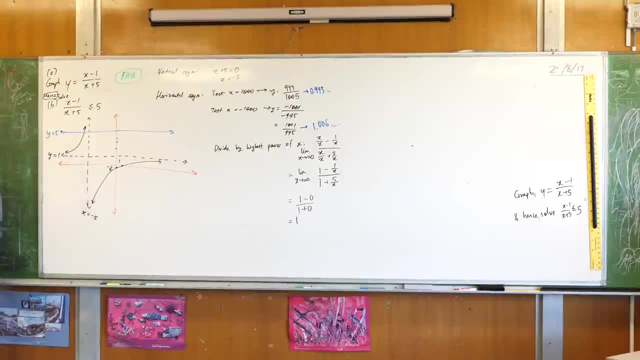 here's five. there's y equals five. so what I want is which parts of this graph are less than or equal to this blue line? okay, good, so you can see this guy over here. this guy is fine from here, and you notice I put a filled circle because the boundary is included. so from here, all the way down here, that's all good, right. so I need to know what that x value is that corresponds to that. I'll come back to here in a minute. 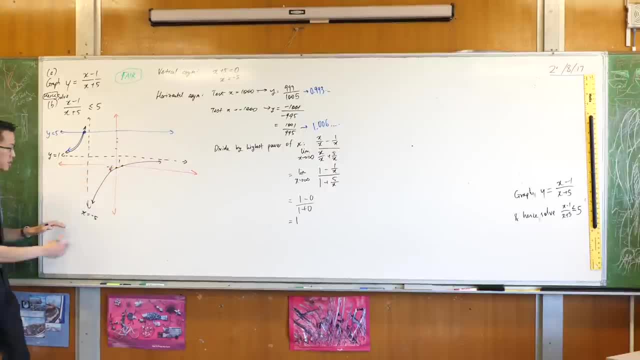 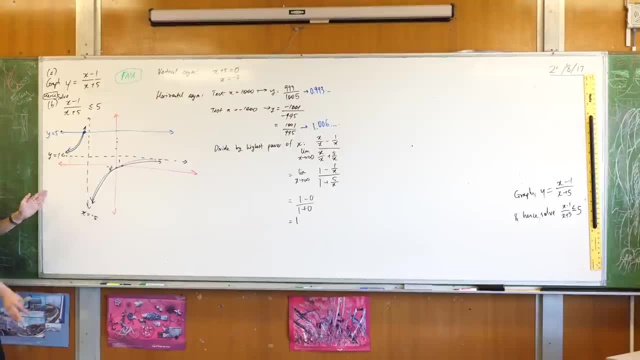 to the right of this. all of that is okay as well. Let's see how far we can get. Let's find this value: When is the graph actually intersecting with 5.? So what I'm gonna have to do is say x minus 1 on x plus 5.. This graph hits: 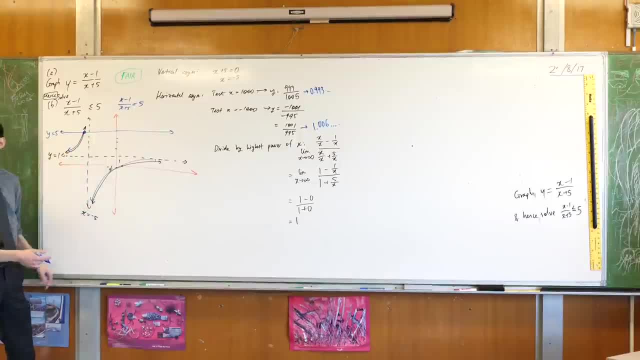 5, at a certain point It equals 5.. That's the boundary right. So therefore I can say x minus 1 is 5x plus 25.. Yeah, so therefore, let's see 4x is equal to subtract 25, negative 26.. So x looks like it's going to be negative. yeah, 13 on 2..